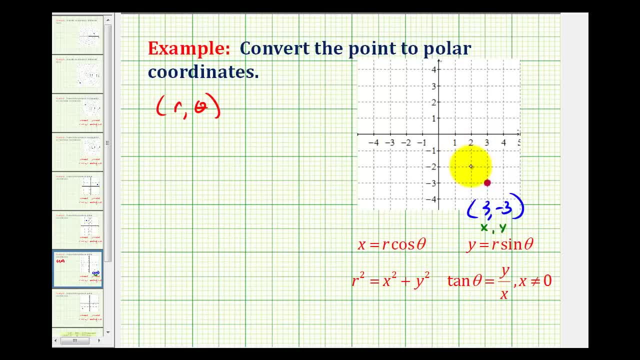 If r is positive, that means the terminal side of the angle would have to pass through the given point, So the terminal side of theta would have to be here. So it's often helpful to sketch a reference triangle to visualize what's happening here. 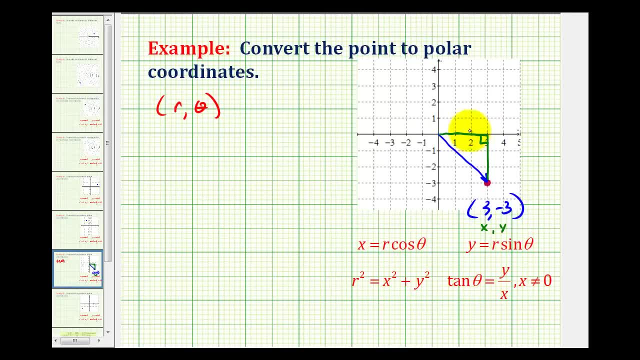 So this would be our reference triangle. We would label this theta: This side of the reference triangle positive three And this side, negative three. Now you may recognize this reference triangle as a 45-45-90 right triangle, which it is. 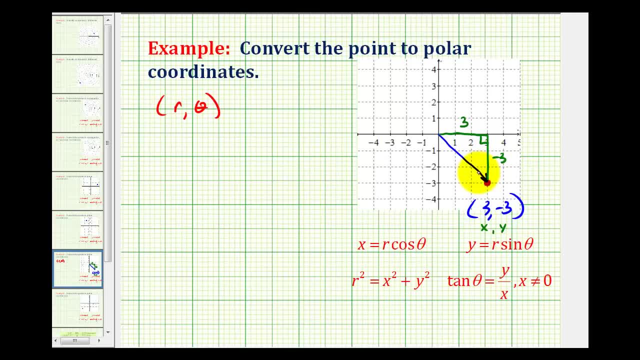 But we're going to assume we don't recognize this and go ahead and determine r and theta using the formulas. So again, if we want the least positive angle for theta, it's going to be the angle that has the initial side here and the terminal side here. 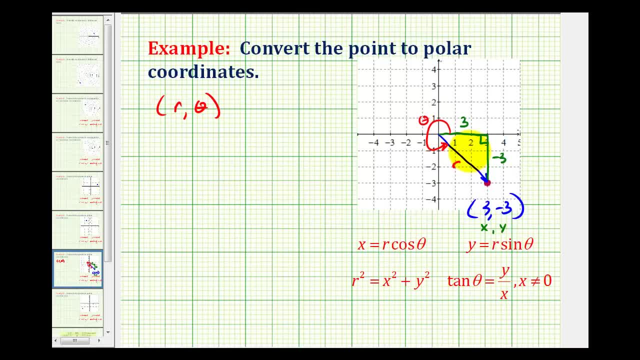 And then r is going to be the length of this hypotenuse. So to determine these angles, we have these formulas that can help us. We have: r squared equals x squared plus y squared, which is just the Pythagorean Theorem. 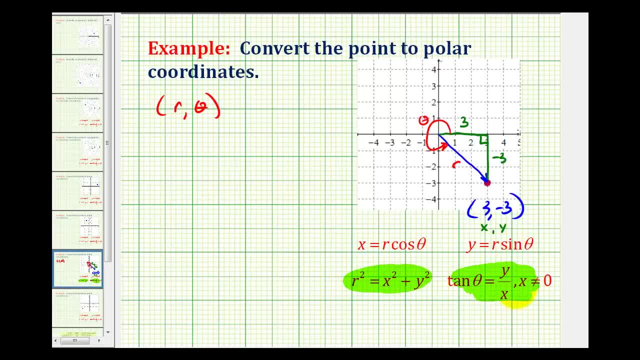 And then we have the equation: tangent theta equals y divided by x, as long as x doesn't equal zero. So we're basically solving this problem using right triangle trigonometry. Let's start by determining the value of r. We know that r squared must be equal to x squared plus y squared. 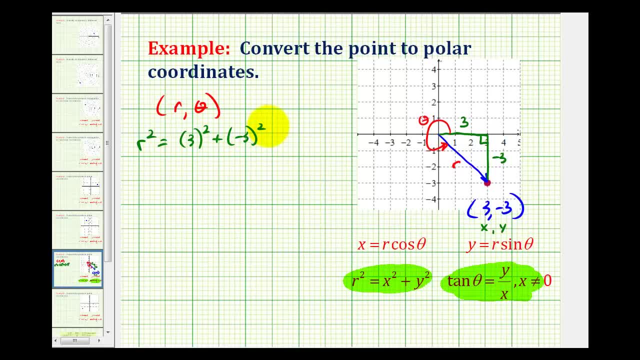 So we'll have three squared plus negative three squared, So we're going to have r squared equals nine plus nine, that's eighteen. So now we can square root both sides of the equation. This is going to give us r equals. well, eighteen is nine times two. 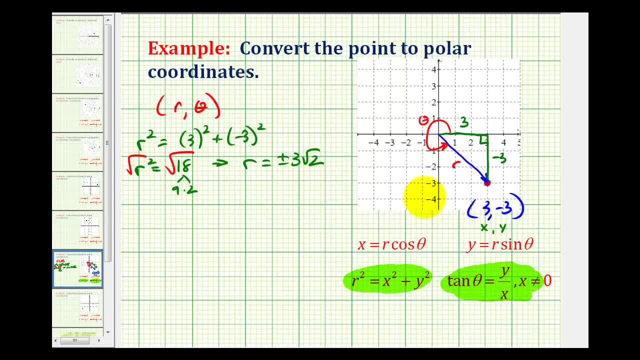 So this will be plus or minus three square root two, And since we're trying to use a positive value for r for our polar coordinates, we're going to use positive three square root two for r. Now we're left to determine theta. Now let's go ahead and determine theta. 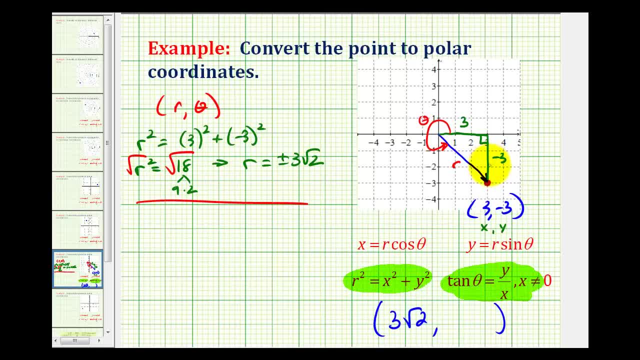 Again, we should recognize theta based upon this isosceles right triangle, but we'll assume we don't. We know that tangent theta would be equal to y divided by x. Well, y divided by x would be negative three divided by three or negative one. 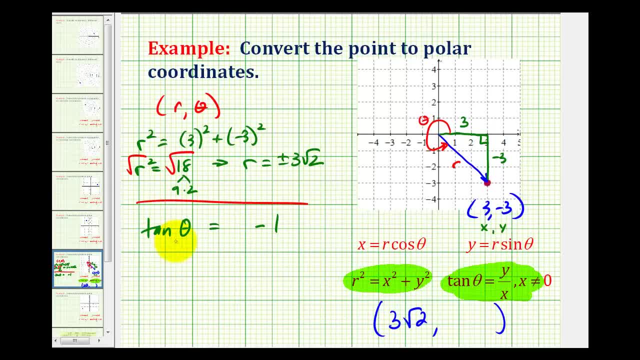 So if we take the inverse tangent of both sides of the equation, theta would be equal to inverse tangent of negative one. Let's go to the calculator and see what angle this gives us. First step is to check the mode. Let's change the mode to radians. 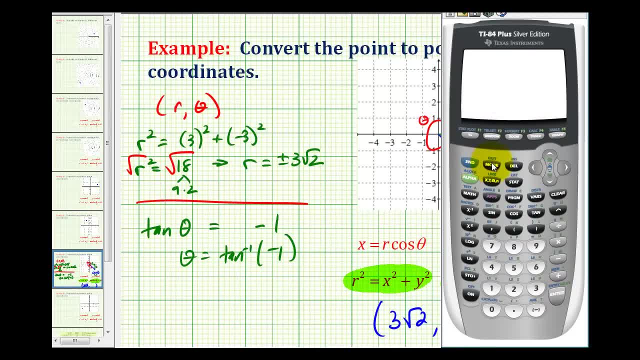 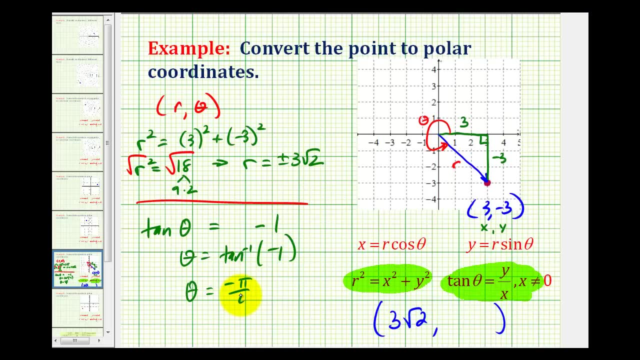 Press enter. Go back to the home screen. Second tangent negative one. Now you might not recognize this, but this is actually negative: pi over four radians. Let's go ahead and write this down and then we'll take a look at our sketch again. 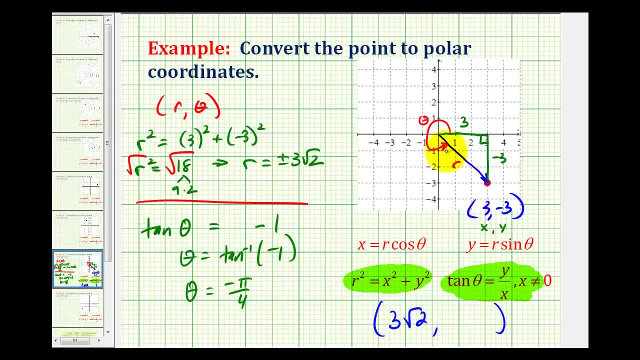 Now negative pi over four radians would be a correct angle for theta. Notice how the terminal side would pass through the given point. But if we really want to have the least positive angle for theta, that would be three hundred fifteen degrees, or in radians that would be seven pi over four radians. 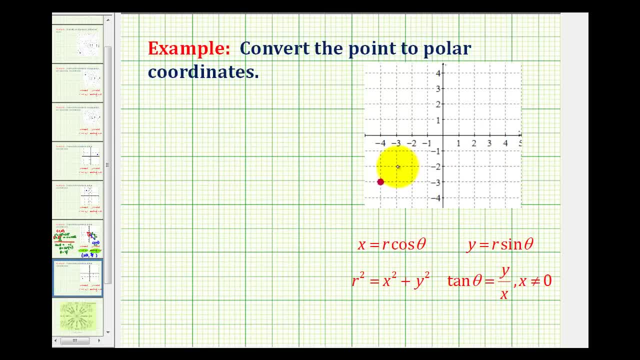 Let's go and take a look at a second example. The given point in rectangular coordinates would be negative four, negative three. And again, let's go ahead and see if we can use this as a positive value for r, which means the terminal side of theta would have to pass through this point. 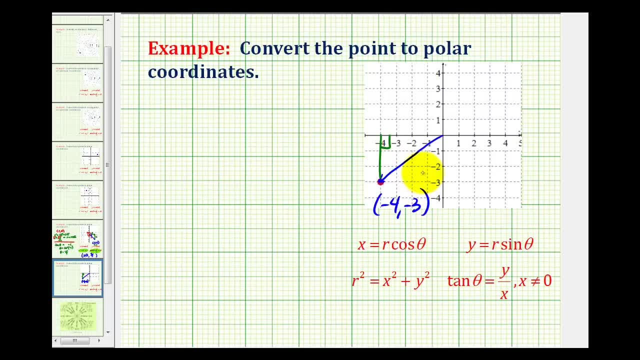 So this would be our reference triangle. Or we would label this leg negative four, this leg negative three, and this would be r, And again we're trying to determine r and theta for this point, given in rectangular coordinates. So we have r, squared is equal to. 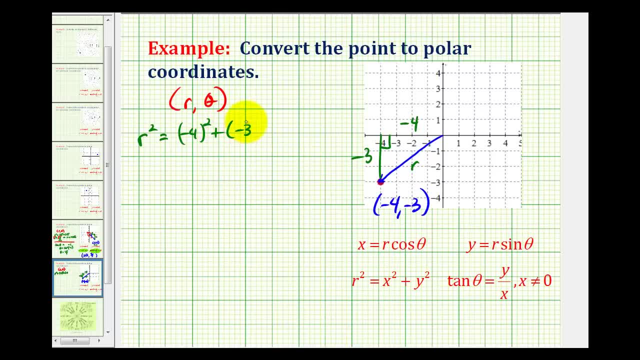 negative four squared plus negative three squared, So we have: r squared is equal to sixteen plus nine, that's twenty-five. Well, this one comes out nice. We have: r equals plus or minus five. Again, if we want to use a positive value for r, 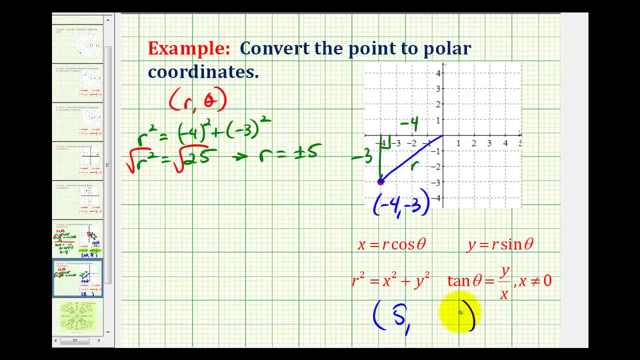 then we're going to use positive five, And then, if we want theta to be the least positive angle, that would be this angle here. Well, let's use our trig equation- tangent theta equals y divided by x- and see what the calculator gives us.